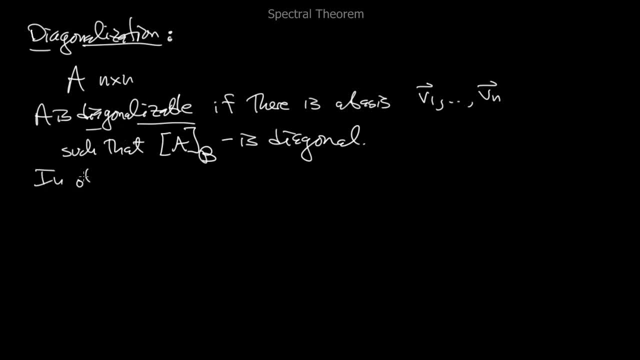 mean. Well, that's just the same thing as saying that, in other words, this basis that I've found is a basis of eigenvectors. So you say a matrix is diagonalizable If, and only if, it has a basis consisting of eigenvectors. All right, we've talked. 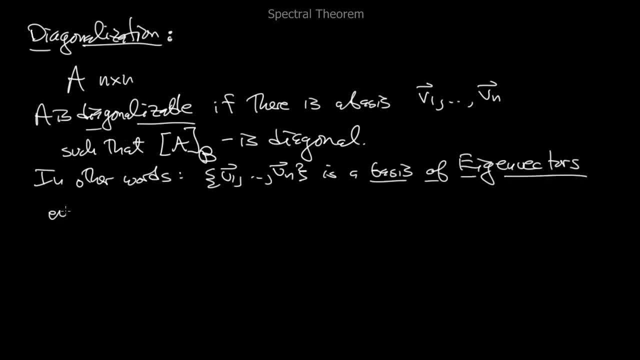 about that several times now. And if the eigenvalues are lambda 1 through lambda n, then what we're saying is that in this basis the matrix becomes lambda 1 through lambda n, and this matrix S is given by taking the vectors v as the column. 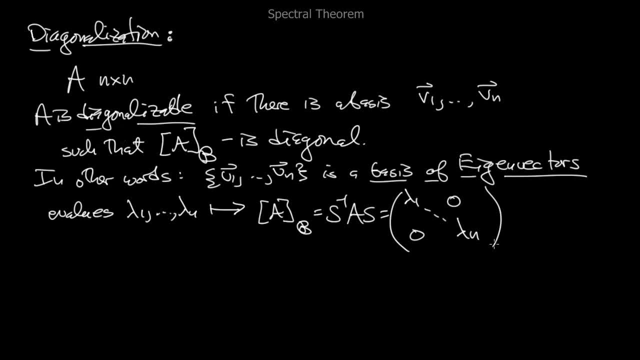 Okay, So that's basically a quick recap of what we've been talking about, And today's sort of theme is that diagonalization is good. It's great when a matrix is diagonal, It's the easiest matrix to understand, And this matrix is. 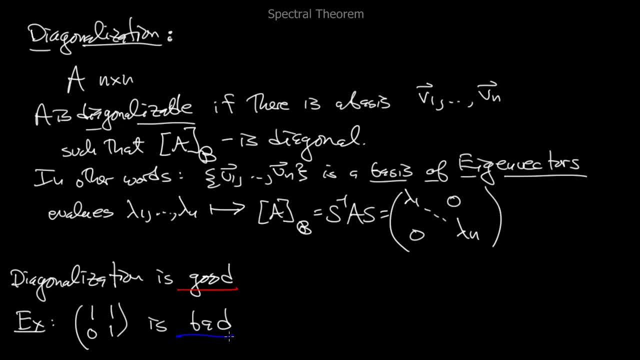 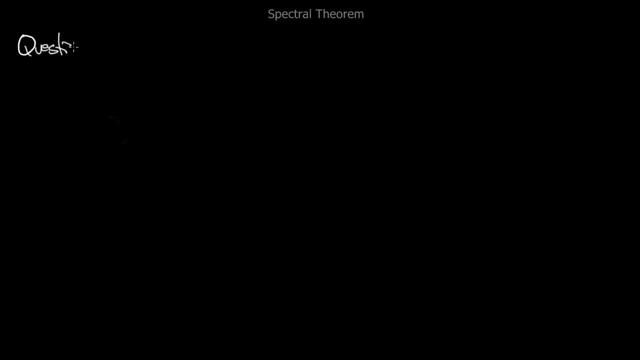 bad because it's not diagonalizable. And what we'd like to discuss is setting what is diagonalizable, And what we'd like to discuss is setting what is diagonalizable, So that's where we can be sure that our matrices are diagonalizable. So the question is when? 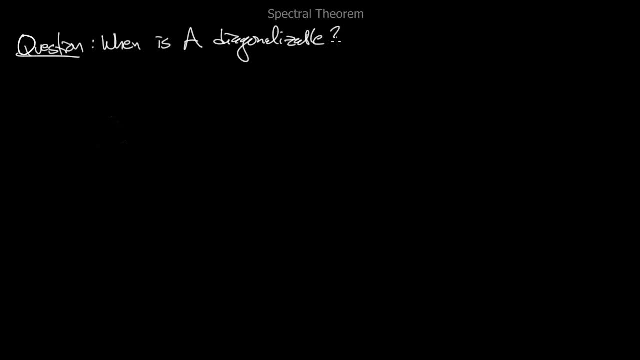 is a matrix, diagonalizable And, as I said, it can be hard to tell. If it has distinct eigenvalues, then it is, But if it doesn't, it can be a fair amount of work to determine whether it's diagonalizable And what the spectral theorem in today's lecture is about. 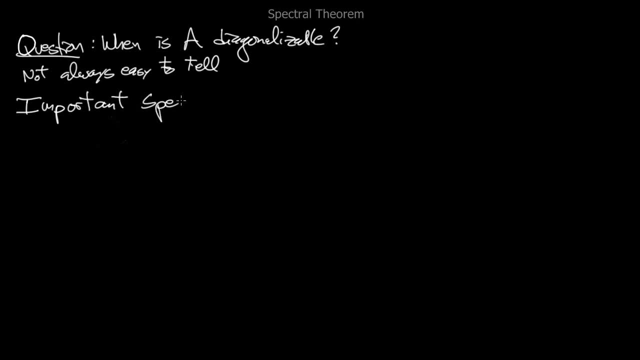 is a special class of matrices which are automatically diagonalizable. So this is a very important special case and I will state it first, as theorem version 1 is the following: Suppose A is symmetric, then it's automatically diagonalizable. All symmetric matrices are diagonalizable. That's a very 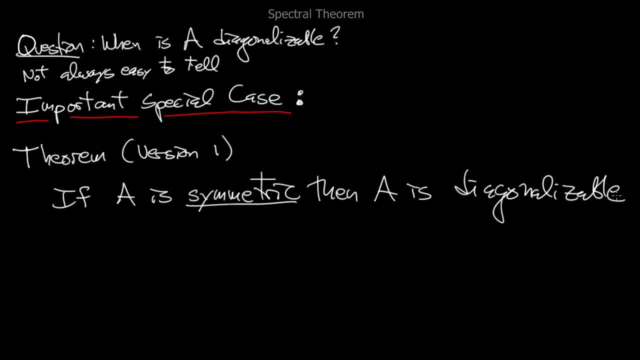 important fact, and I'm just stating it here, just like that. In a little while, I'm going to have a stronger version of this theorem with more information in it There's. you can say quite a bit more than this, but the starting point is this. 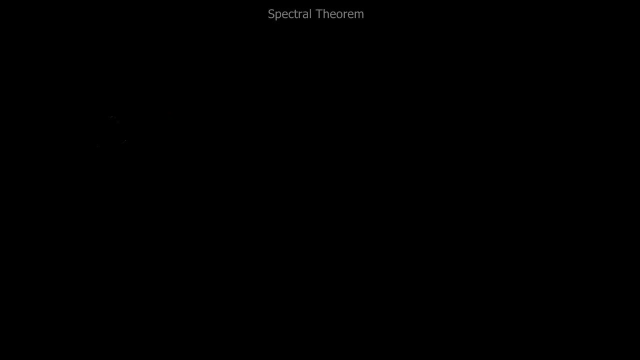 basic fact that every symmetric matrix is diagonalizable. Okay, so let's just do a couple of quick examples. Let's take a A to be a diagonal matrix with zeros on the diagonal. Well, let's see, the characteristic polynomial of this fellow is lambda squared minus A squared which. 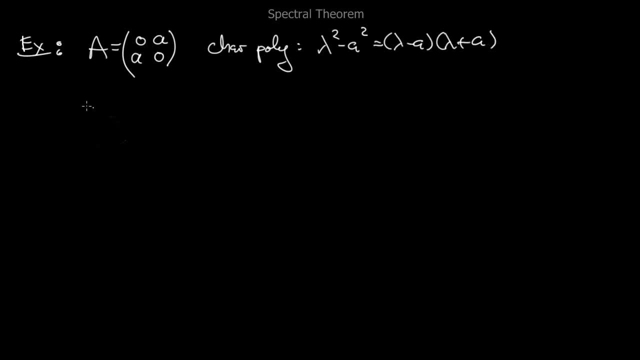 is lambda minus A times lambda plus A, and that certainly has two distinct eigenvalues, A and minus A, unless A is zero, of course, in which case the matrix was just zero, which is fine too. So all of these matrices are easily seen to be. 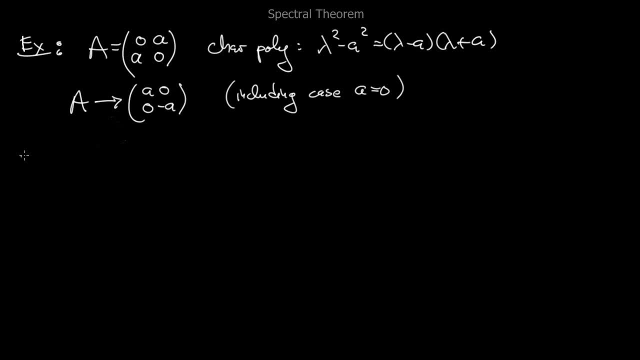 diagonalizable. Let's do another simple example. Suppose I gave you a two by two matrix like this, where I just took some number A and I hand: all four entries were equal to A. Well, let's just see if we can diagonalize it. The characteristic: 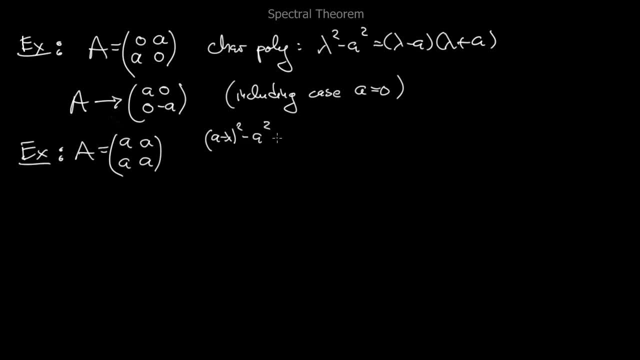 polynomial is A minus lambda squared minus A squared, which is lambda squared minus 2A. lambda plus A squared minus a squared and those cancel and you get lambda squared minus 2a lambda and that factors as lambda times lambda minus 2a and the solutions of that are: 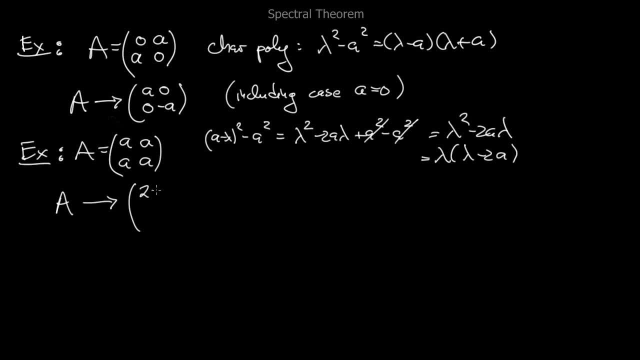 the two numbers 0 and 2a, and again they're distinct, unless of course, a is 0, in which case you just have the 0 matrix. so again, all of these are diagonalizable. now note the trace of this matrix: AAAA is 2a and the 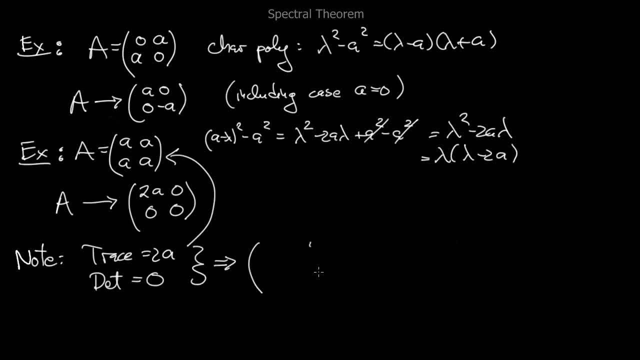 determinant is 0, so you can actually read off this diagonalization without even doing it much work. it's a matrix with determinant 0, so it has to have a 0 in it, and then the trace has to be 2a, and so it's very easy once you know it's. 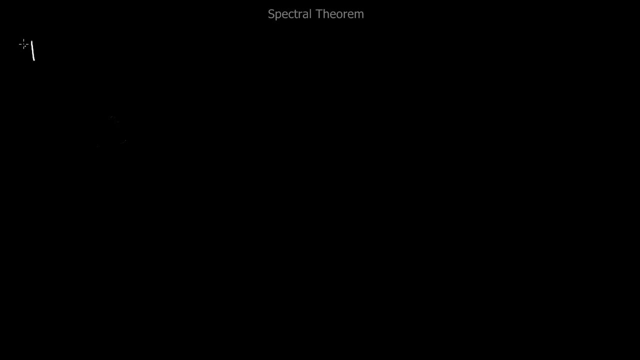 diagonalizable. you just compute the determinant and the trace, and it's often quite easy to see what a diagonalization is to Okay. so here is the more robust version of the theorem which has more information in it. So suppose we're given an n by n matrix- excuse me, symmetric. 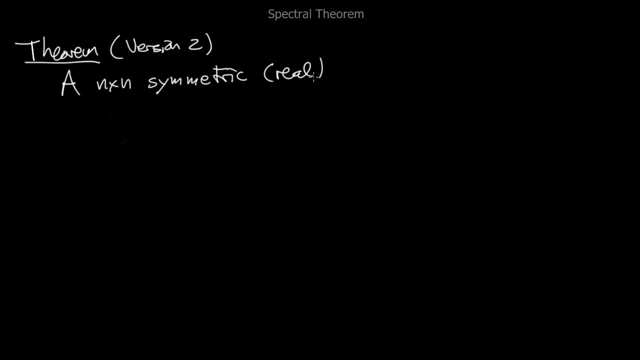 matrix A and I'll emphasize, it's a real symmetric matrix. here, then, the first statement is that all of the eigenvalues of A are real. This is very important to you. you cannot have complex the. the eigenvalues are real, you don't. 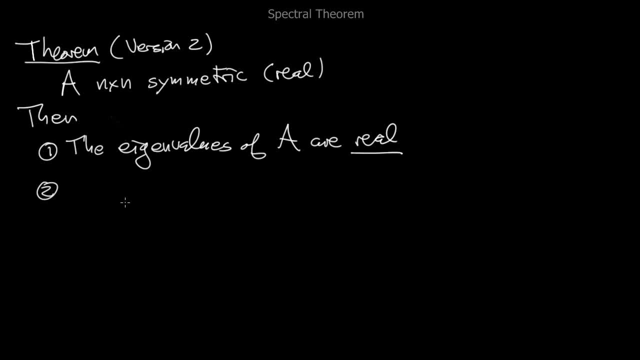 need complex numbers to find the eigenvalues. Secondly, the eigenspaces are orthogonal. that is to say, if you have an eigenvector v and eigenvectors v and w with different eigenvalues, then v and w are orthogonal to each other. so 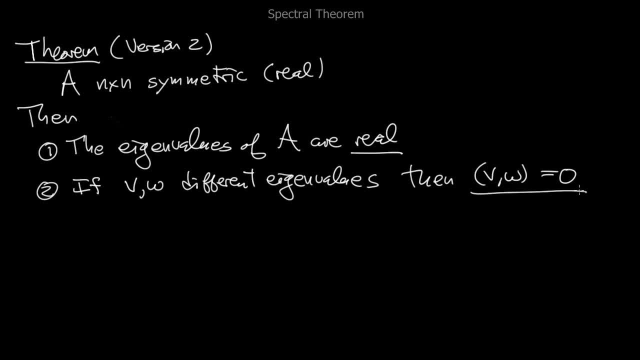 distinct eigenvectors, excuse me, eigenvectors with different. the distinct eigenvalues are orthogonal. That's a very nice fact. And finally, you can find basis V1 through Vn of the vector space with the following properties. Well, first of all, 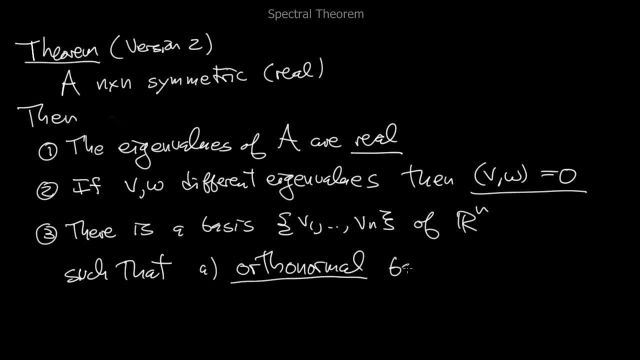 this is an orthonormal basis, So not just any old basis. I can actually find an orthonormal basis which diagonalizes the matrix, which is, that is to say, consists of eigenvectors, which is to say that the matrix, with respect to this basis, is diagonal with these real. 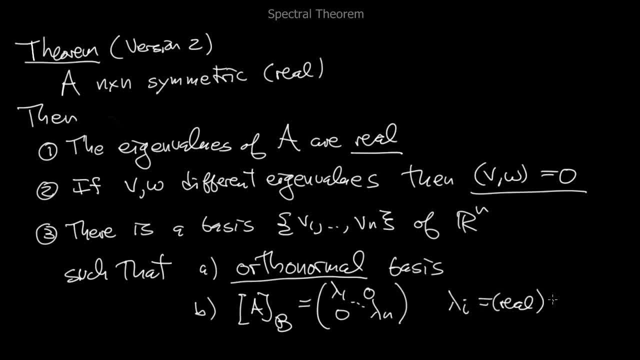 eigenvalues down the diagonal. So that's extremely nice. There's a lot of nice properties here. You have an orthonormal basis, the eigenvalues are real, the distinct eigenvectors are orthogonal. It's a lot of sort of nice structure. 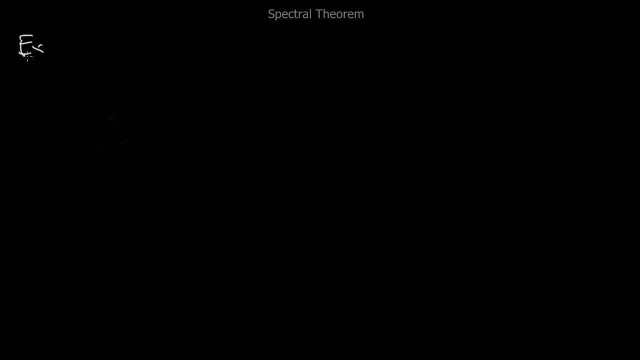 It shows you that symmetric matrices behave pretty nicely. So let's do a quick example. Let's go back to our example like this. Let's see what are the eigenvectors. Well, we saw there were two eigenvalues A, and a moment's thought tells you that for the A eigenvector. 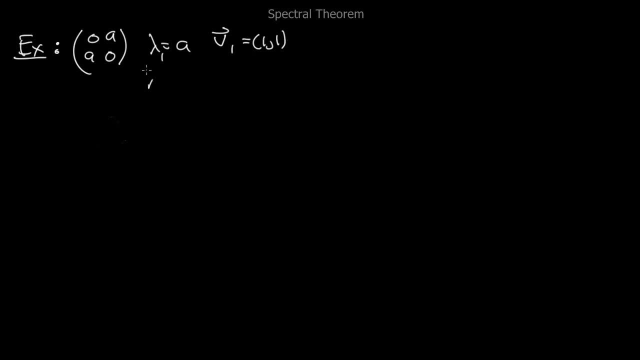 you can take the vector and the other eigenvector is: eigenvalue is minus A and that means, and for that you can take the eigenvector, and indeed these are orthogonal. So there's an orthogonal basis and you just have to normalize it. 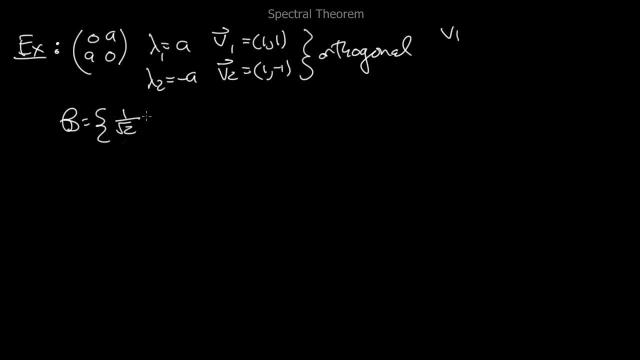 to make it orthonormal, You take the basis 1 over radical 2, 1, 1, and 1 over radical 2, 1, minus 1.. That's an orthonormal basis of the space consisting of eigenvectors and which diagonalizes this matrix. Okay, let's take 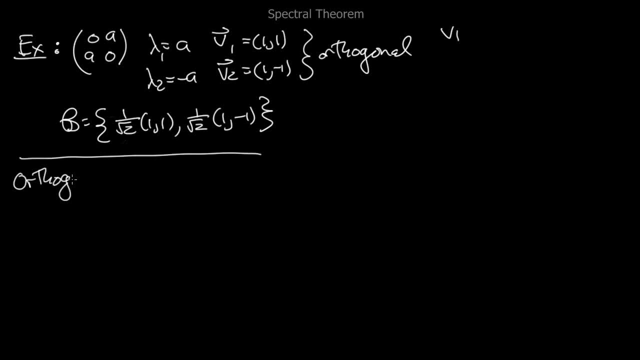 a quick look why this all works. What makes it work? It's actually quite simple. Let's look at this orthogonality property. So suppose you have an eigenvector V with eigenvalue lambda and another eigenvector with eigenvalue 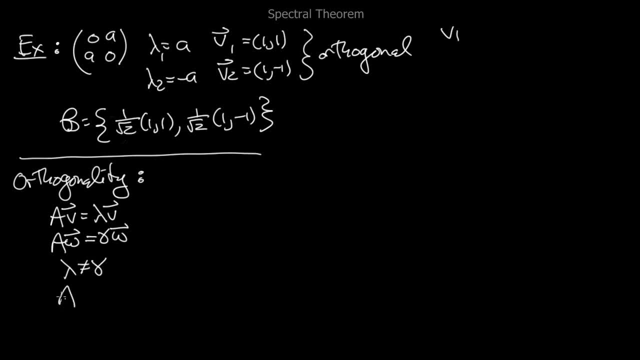 gamma, and suppose lambda and gamma are not equal and that A is symmetric. From this I'm going to conclude that V must be orthogonal to W very easily. So let's take this inner product. I'm going to write down, Write it this way: V- inner product. W is just the ordinary dot product and go. 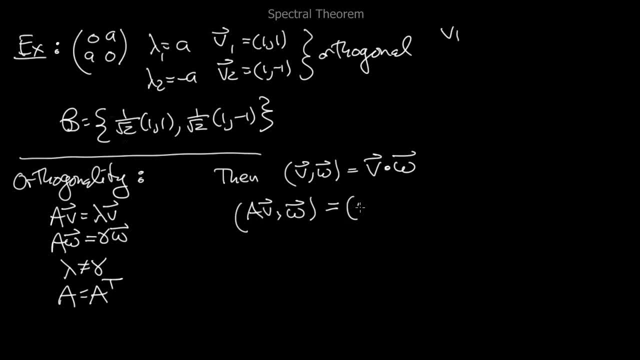 back to the section on inner products and you'll see that that satisfies this property. AVW is the same thing as VA, transpose W. We've seen that a number of times, and now A transpose is equal to A because it's symmetric. So here you have. 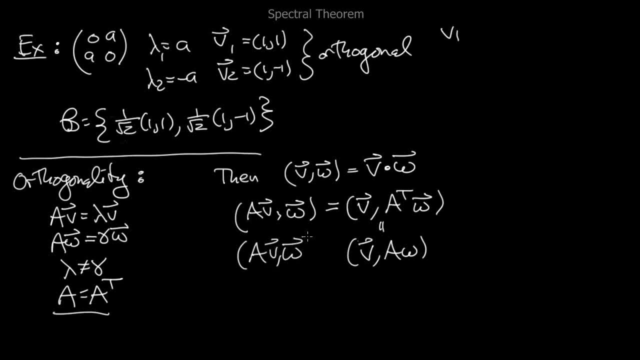 V, AW. and now let's see: V has eigenvector lambda, so you can pull that down, and W has eigenvector gamma, and now this is a bilinear inner product, which is to say the lambda and gamma pull out, So you get this equality and now you're home free. Look at this. If 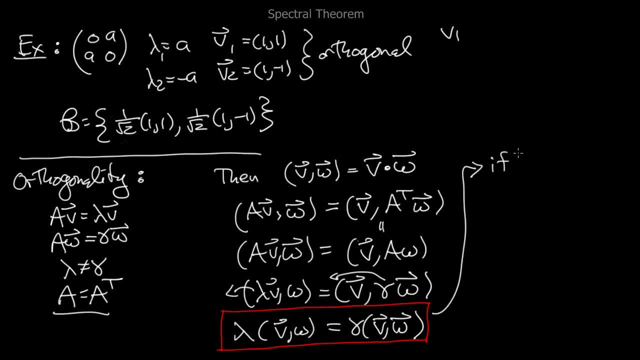 VW is not zero. well then you could cancel it. right, and if you cancel it you would conclude that lambda equals gamma. but I told you that lambda is not equal to gamma, right here. so they can't, that can't happen, that's a contradiction. so it must be that VW is zero, because then this: 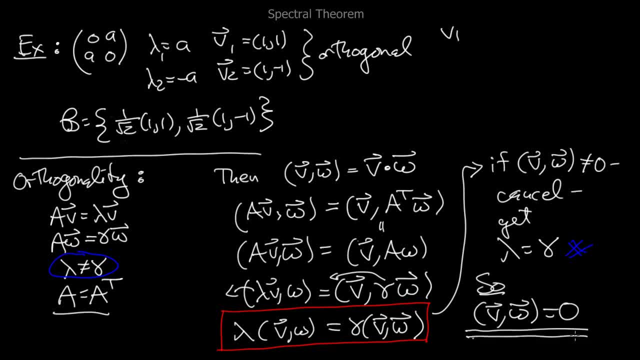 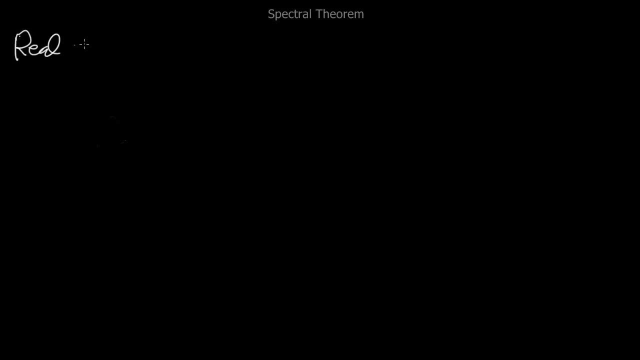 equation doesn't lead to a contradiction. it just says zero is equal to zero, so VW is equal to zero. they are automatically orthogonal. it's just a very simple property of inner products and transposes and such and the the fact that the eigenvalues are real is very similar. let's just 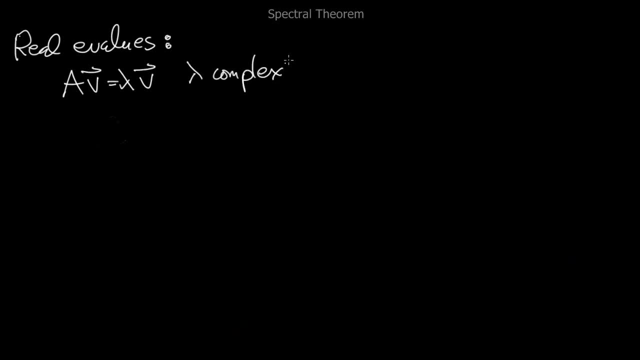 write that down. suppose V has eigenvalue lambda, which might be a complex number, and i'm going to show that in fact it has to be real. so let's pass to the complex numbers to do this calculation and let's define the complex inner product or hermission number. 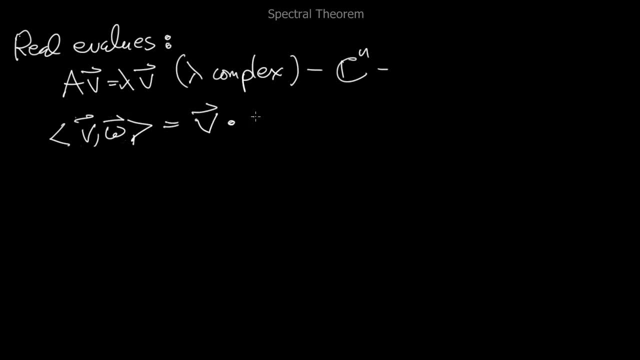 interproduct on Cn. We've seen this before where instead of vw you take vw bar, And this is sometimes called the Hermitian interproduct- And it satisfies if you take Avv, just like before. you get Va, transpose v, except you also get a bar on the A. But now let's see. 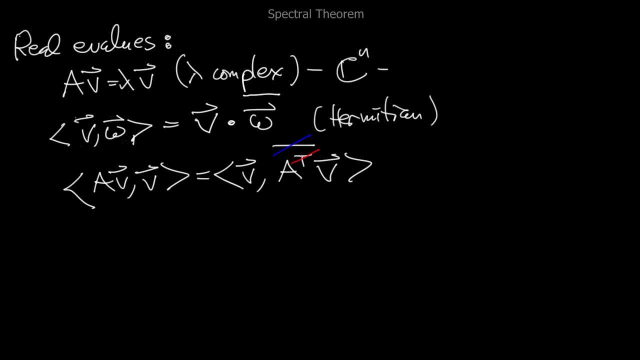 A is symmetric, so the t goes away and A is real, so the bar goes away. And so you conclude that Avv- over here, is lambda vv and over here is v- lambda v because of the eigenvalue. Now the lambda pulls out on this side And, the crucial thing is, because of the bar. on the second term, 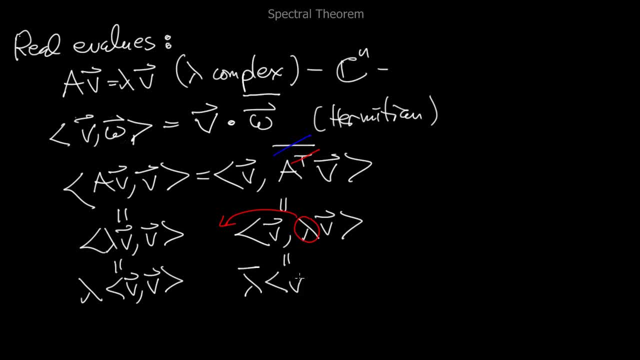 this pulls out with a bar. That's the crucial point. And over here you get lambda bar vv. So I've concluded that these two things are equal. But if v is not zero, then the interproducts are non-zero and you can cancel. 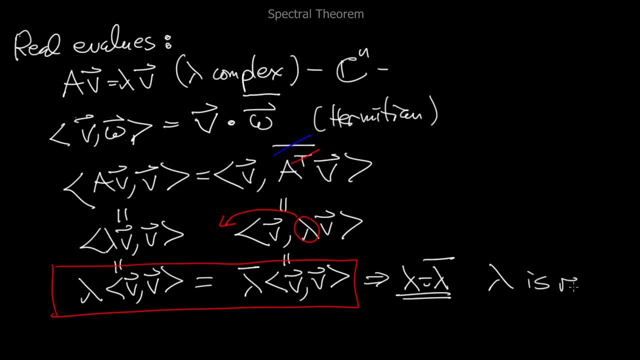 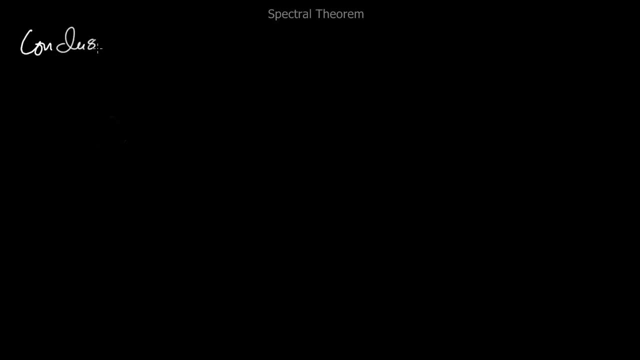 them, and you conclude that lambda must equal lambda bar, That is to say, lambda must be real. That's all there is to it. So that's why the spectral theorem is true. That's most of the proof of the spectral theorem, And so the conclusion is- I'll just remind you of the- 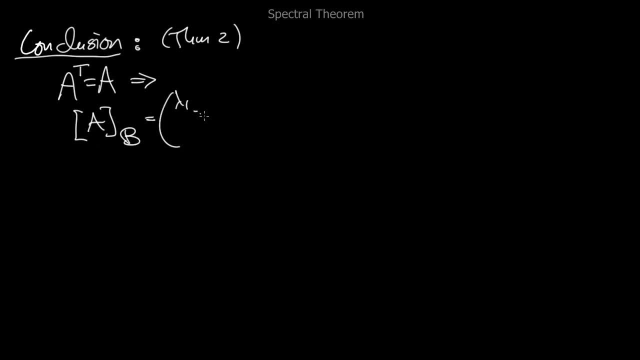 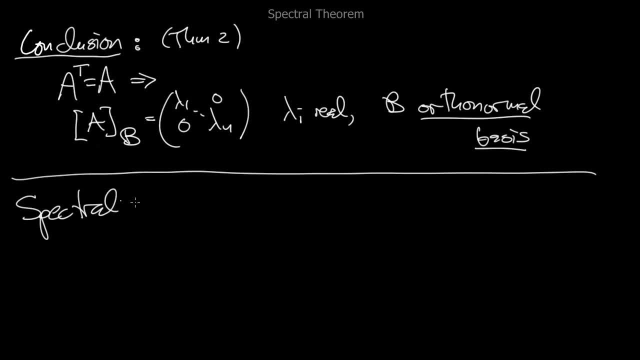 And I'm going to go back to the theorem, And I'm going to go back to the theorem, And so I'm going to go back, and, and I'm going to go back, and the spectrum says the following: You start with a, an, n by n, real symmetric matrix. 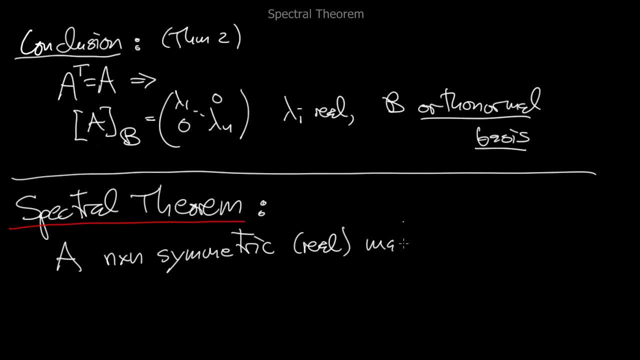 Then the assertion is that you can find a, then you can write A as a integral. but you can also Figure out the y-axis urائ s, Yo, b, Thi, a, a. a is equal to Q, D, Q inverse, where D is diagonal with real eigenvalues and Q is 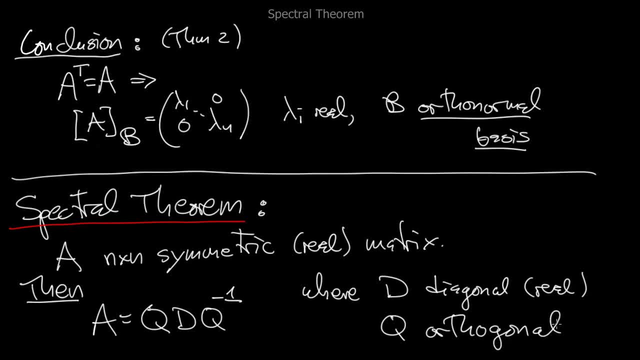 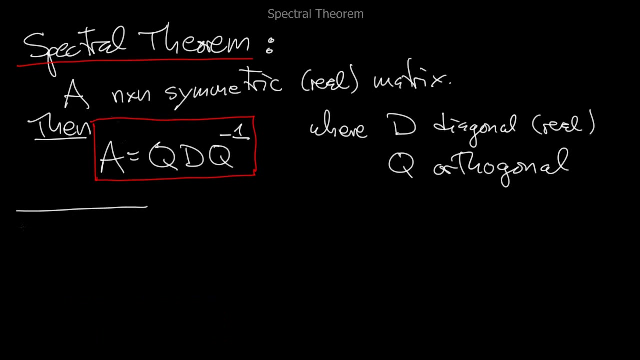 orthogonal. okay, so a can be diagonalized. that's the first statement. and not only that, it can. you can use an orthogonal matrix to do it. and this is the sometimes called the spectral decomposition of a, writing it as Q, D, Q inverse. so in other words, if you want to remember the spectral theorem in the 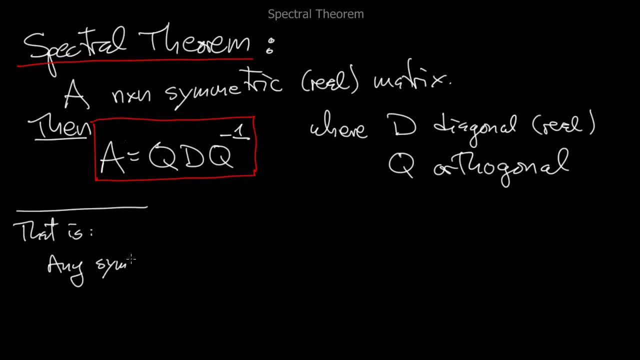 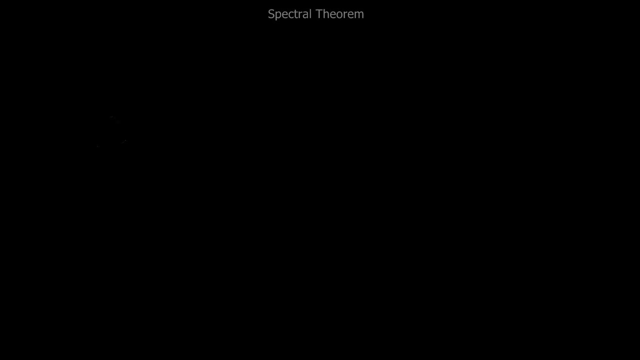 phrase what the spectral theorem says, that any symmetric matrix can be diagonalized by an orthogonal matrix. okay, that's just another way of saying the same thing. the orthogonal matrix is Q and the diagonalized matrix is D. okay, so why is this true? well, we've practically said it already. 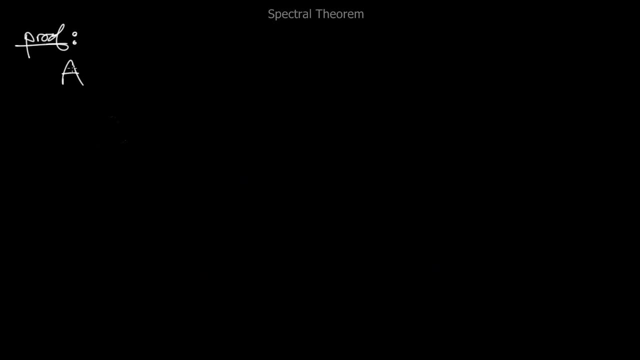 let me just say it. so you have a symmetric matrix A, and I told you we can find an orthonormal basis such that A, with respect to this basis, is diagonal. that was the second version of theorem 2. well, that's, that's it. that's all you. 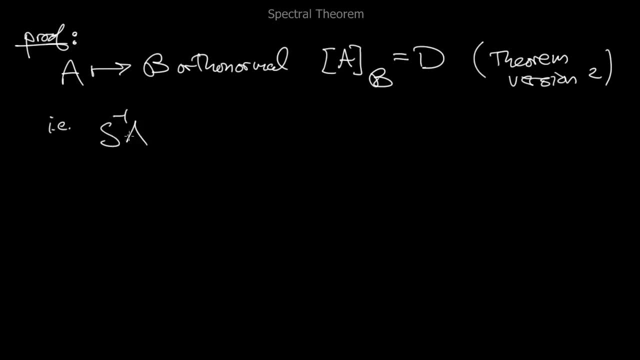 need really, because what does this say? well, make this. this says that S inverse A, S is D, where S is the matrix, the you make out of the vectors V and the fact that the basis is orthogonal. excuse me, orthonormal is exactly, it's if, and only if S is orthogonal, that's. 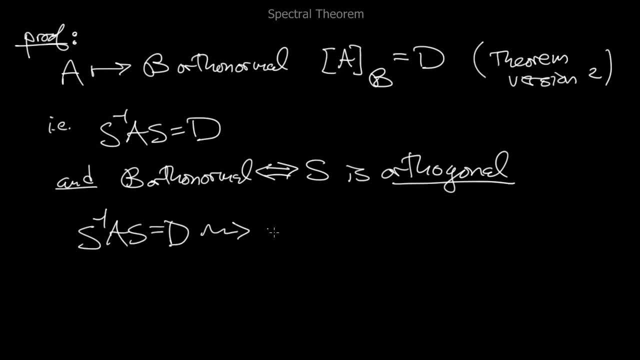 we've seen that a number of times. so that is to say, S inverse, A, S is equal to D. or if you bring the S to the other side, you can write: A is equal to S, D, S inverse. and well, in the theorem I just took it, Q is equal to S, S is orthogonal. 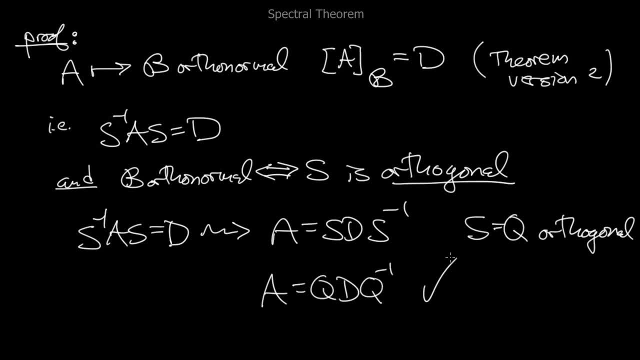 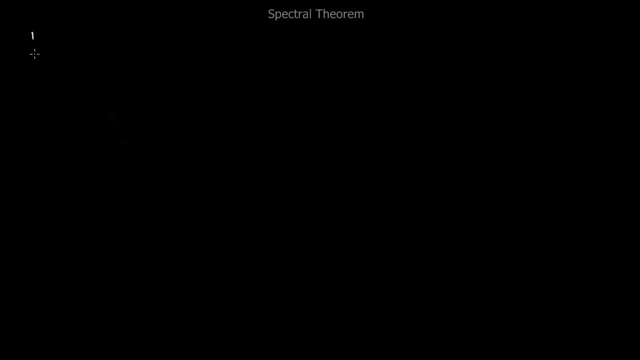 and so I write: A is equal to Q, D, Q inverse, and that's the theorem. so it's really nothing more than version 2 of the theorem, where you bring the change of basis matrix into the picture. okay, so let's do a couple of examples. let's take 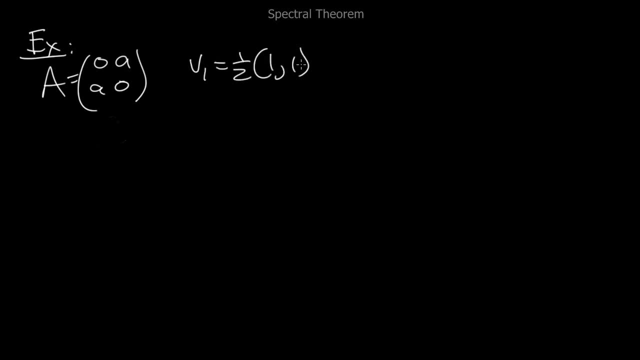 my matrix like this. I saw I could choose my orthonormal basis to be like this, and so I take Q to be. I make V1 the first column and I make V2 the second column, and then I have that Q inverse A. Q is going to be diagonal. let's check if I write down Q. 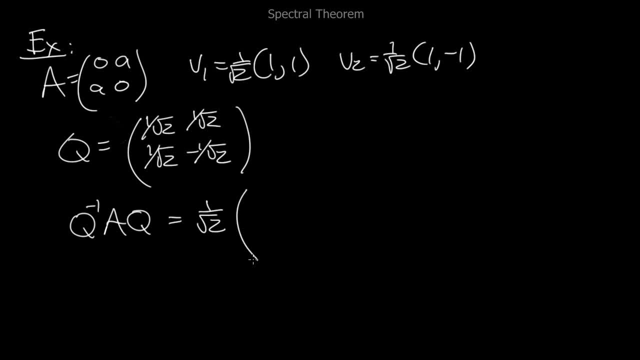 inverse A Q. let's see Q inverse. I'll let you check that. that's like this: actually Q inverse is equal to Q, but anyway, that's Q inverse times A times Q. and if you multiply it out, what do you get? you get you can pull the radical twos out.